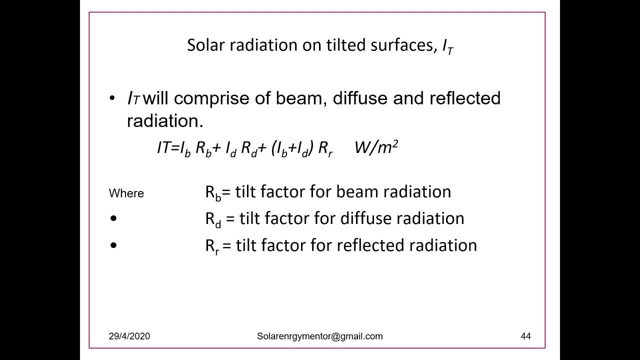 In our last lecture we have seen solar radiation on tilted surface. IT- That is IT, is equal to IBRB plus IDRD plus IB plus IT, that is IG, into RR. So IB is a beam radiation, IT is diffuse radiation and IB plus IDR is global radiation RB- we have just made a mention. 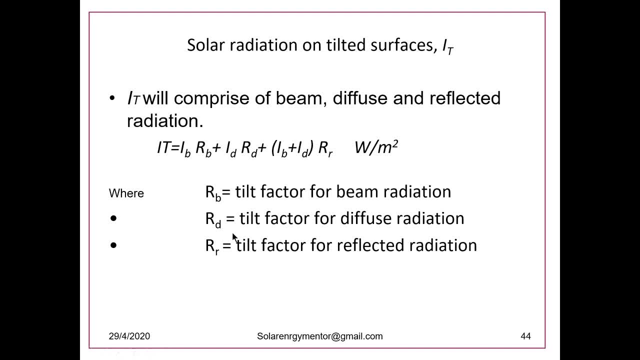 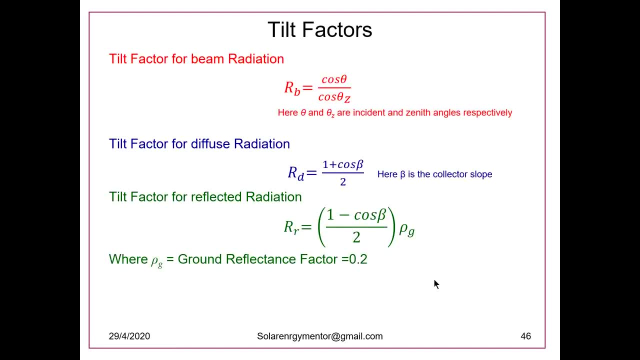 RB is a tilt factor for beam radiation, tilt factor for diffuse radiation and tilt factor for reflected radiation. The expressions for tilt factor are as follows: So tilt factor for beam radiation RB is equal to cos theta by cos theta z. So cos theta theta is the. 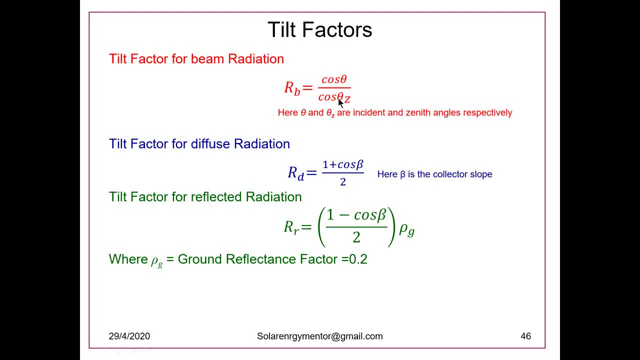 incident angle and theta z is the zenith angle. Tilt factor for diffuse radiation is equal to RR. Diffuse radiation RD is related to slope of the collector, So which is 1 plus cos beta by 2.. Beta is the slope of the collector, or tilt. collector tilt, we can say Then tilt. 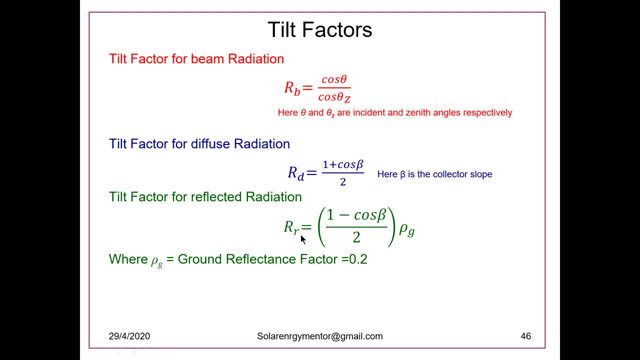 factor for reflected radiation, RR. This is also related to the slope of the collector as well as ground reflectance factor. So it is 1 minus cos beta by 2 into rho g. Rho g is the ground reflectance factor, The value of ground reflective factor, ground reflectance. 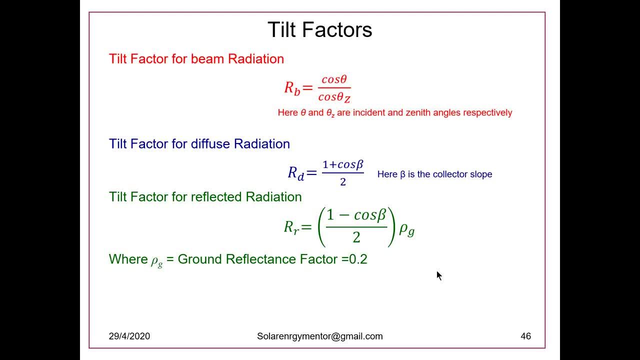 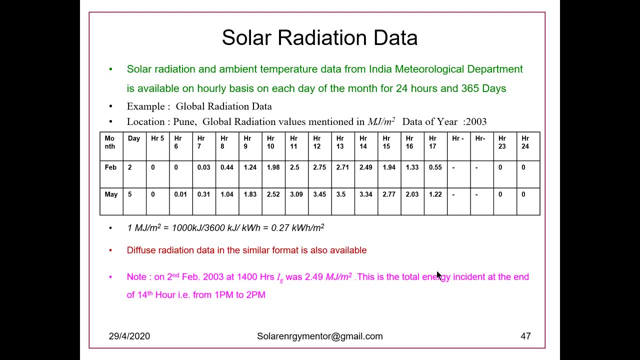 factor is taken universally to be 0.2 at all locations. Now something regarding solar radiation data. How solar radiation data? in what form it is available? So if you apply to India Meteorological Department and request them to spare the radiation data, the radiation. 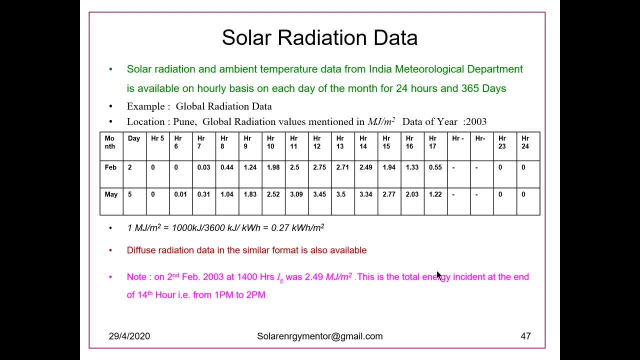 data available will be in this format, So it is for 24 hours and 365 days, So it is hourly data available. For example, this is just an abstract or snapshot of the data available in the format from meteorological department India meteorological department. So, for example, the global radiation data. 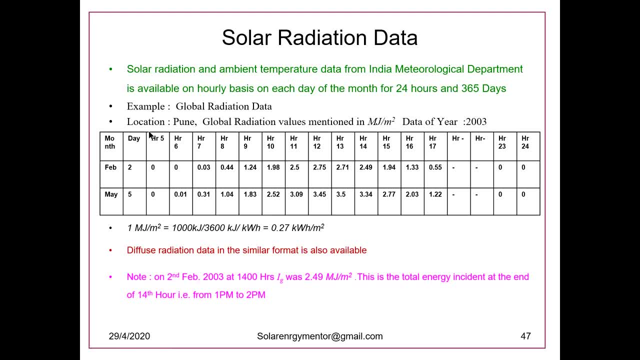 table is different and other tables are different, So this is a global radiation data table. Location For Pune location: Okay, Okay, I have called this data in 2003, so this is global radiation values mentioned in mega joules per meter square. so data of the year is 2003. now you can see here the first column. 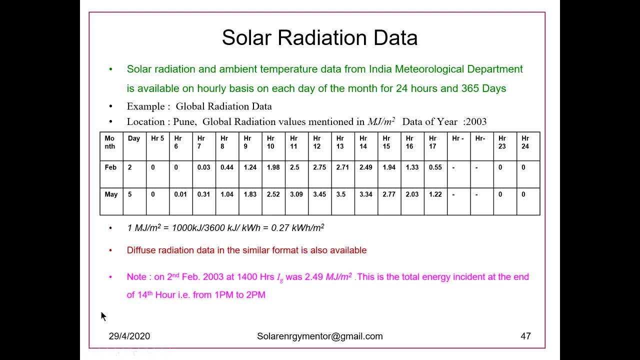 is month, right? so all these months are covered in this data, right from January till December. so January to December, 12 months of data is available, and then for all days, for all days again, like from 1st January till 35th January, February till 31st of December, so all the. 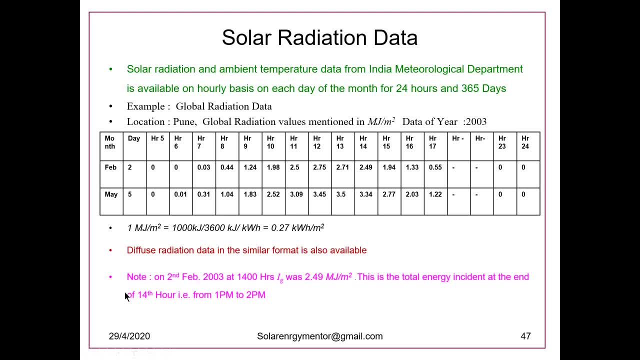 days, like 30- 31 days of the year, so this is 365 days. data is given, then hours, so I have just taken the abstract of two days like February, 2nd February. now the hours are 24 hours, but solar radiation is generally available after 5 hours, so the data available is the readings. 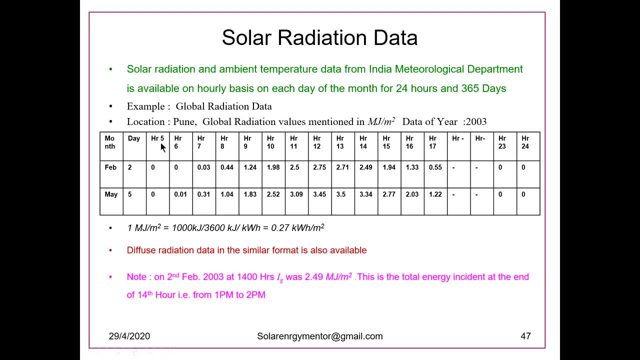 available are from 5 hours, so hour 5 means 5 o'clock, So 5, 6, 7, 8, 9 till 24, like in the midnight. so obviously the midnight or the evening readings are 0 here now. you can see here the February 2 readings, 5 o'clock, reading 0. this is a global. 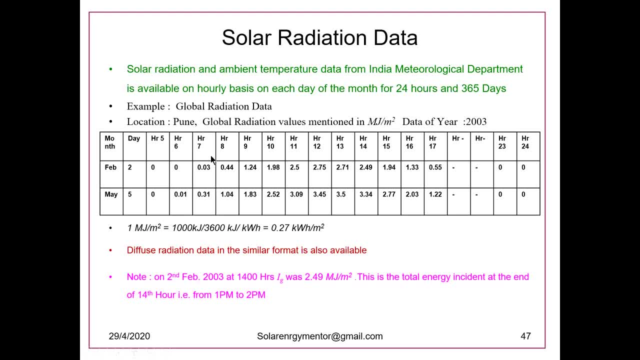 radiation reading. 6 o'clock reading is 0. 7 o'clock, 0.03. 8 o'clock goes on increasing 0.44, 9 o'clock, 1.24, 1.98. this is in mega joules per meter square. 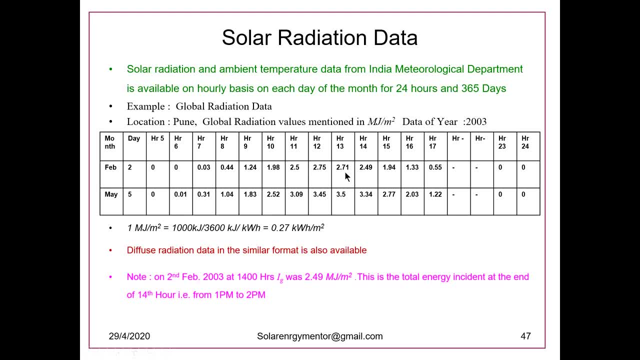 Okay, so it goes on increasing to 2.5, 2.75, 2.. and goes on decreasing after 2.71, and all again may, another day, may. similar trend is shown here. so this is just a is shown to just get an idea of how solar radiation data is available and how we have to convert it for. 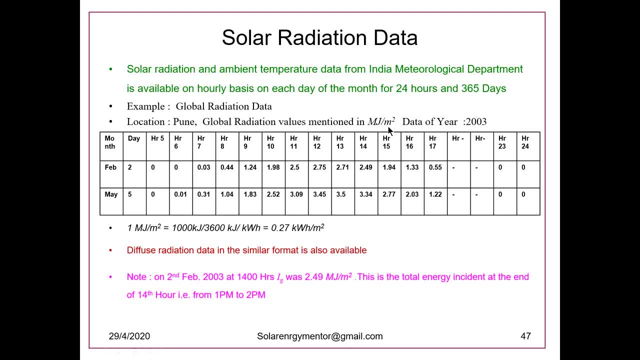 our use now. here data available is in mega joules per meter square. if you want to convert this into kilowatts, This is the conversion: 1000 kilo. 1 mega joule is equal to 1000 kilo joules and 3600 kilo. 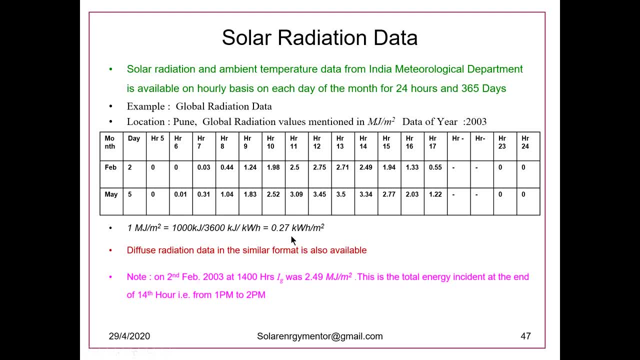 joules is equal to 1 kilowatt hour. so if you divide this you will get 0.27 kilowatt hour per meter square. that is, 1 mega joule per meter square, equal to this diffuse radiation data which I am showing again. a diffuse radiation data in the similar format is also available. 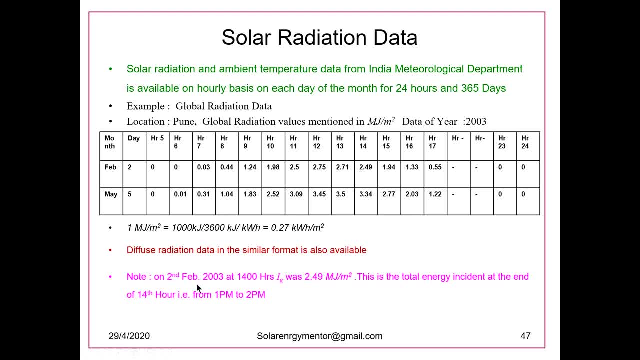 now here. one thing must be noted: that on 2nd of February 2003.. So this is 2nd of query 2003. at 14 hours you can say here: at 14 hours, Ig Global radiation was 2.49 mega joules per meter square. so this is what. what? what this rating? 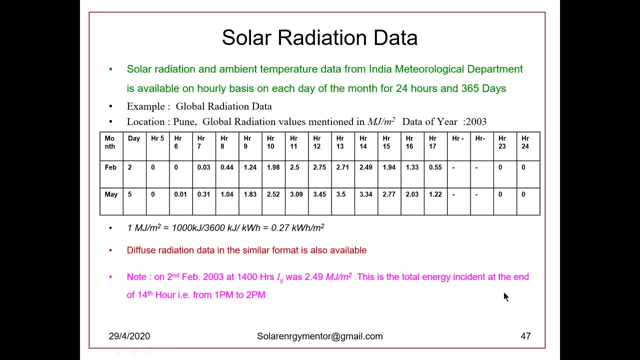 indicates. this reading indicates the energy collected from 1 Pm to 2 pm, Like 13 hours to 14 hours. so in one hour how much energy is connected to the 2.5 a mega joules of energy up significant? 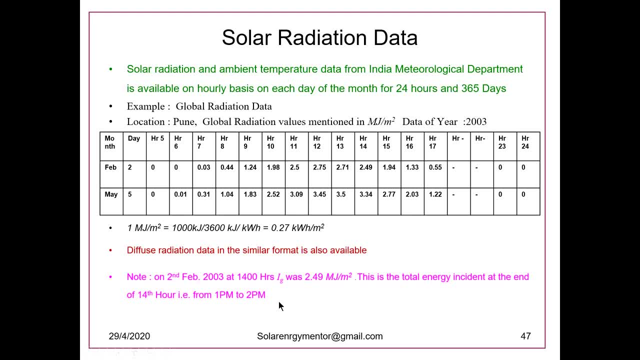 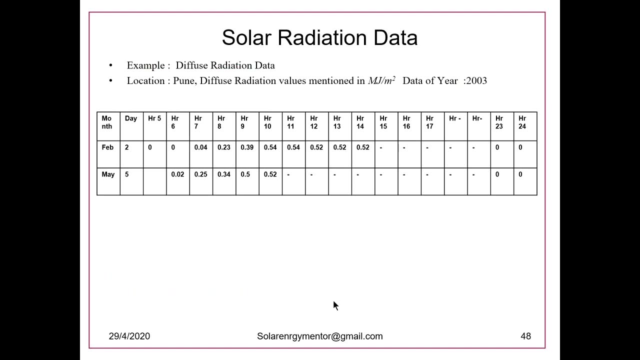 12. 00. 00. square of area. So it is the energy collected in one hour. So this has to be taken into consideration while solving the example or while solving the while estimating the resource available or energy incident on a collector. Now this is diffuse radiation data sample. 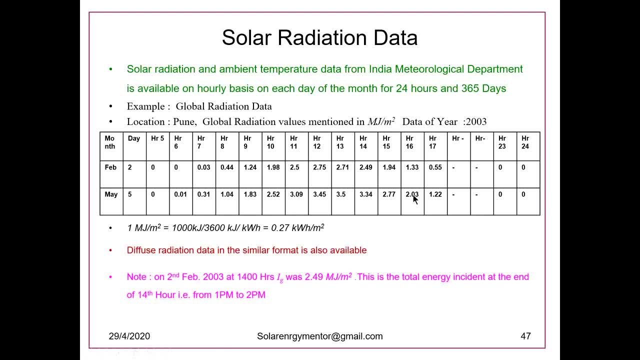 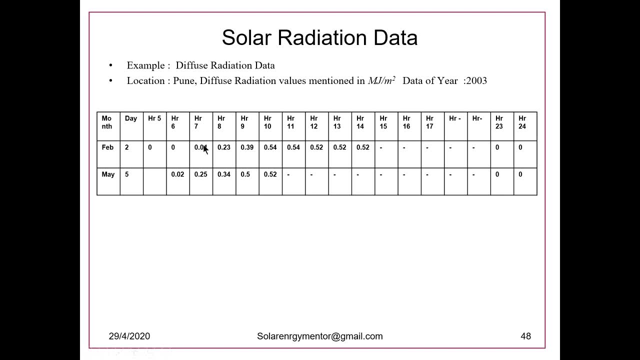 of the diffuse radiation data for the same. for the same you can say period of February to May 5, so February 2 and May 5 diffuse radiation data. obviously, diffuse radiations are less as compared to the global radiations, So 0.04, 0.023 or so, like this these are. 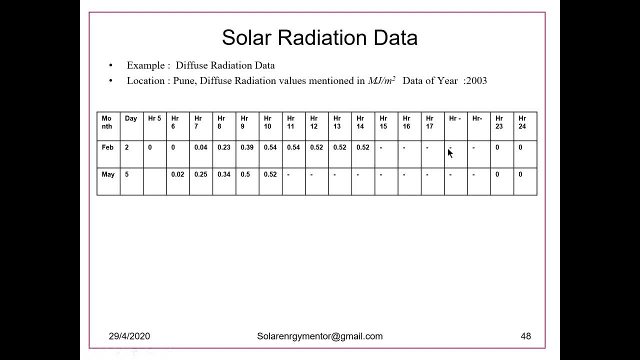 the diffuse radiation These dashes indicate the readings are not available, or maybe the the sky cloudy. due to that, readings are not available. So we can extrapolate these readings, or we can extrapolate from the previous data, So you can also extrapolate. So let me explain this data able. So if this, for example: 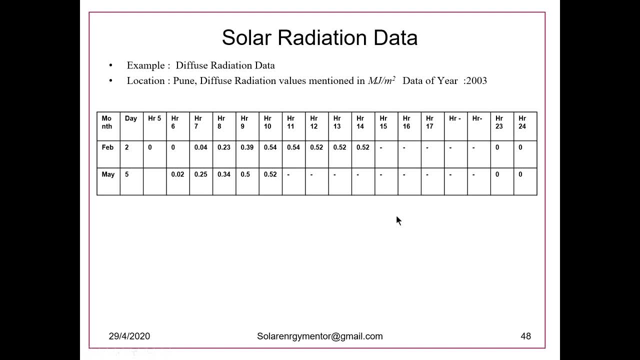 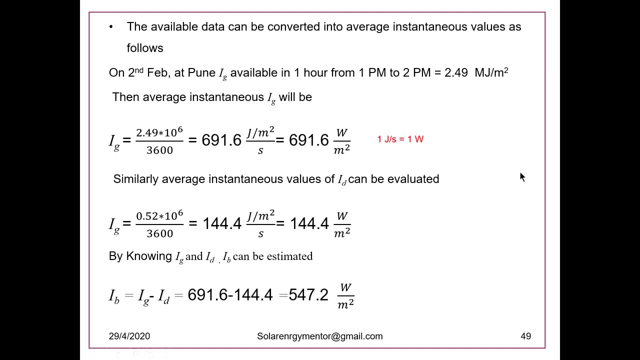 day or the next day, So, but these readings can be. there is no much difference in the readings. So you know, even if the readings are not available, we can easily assume the readings with a close accuracy. Now the available data can be converted into average instantaneous. 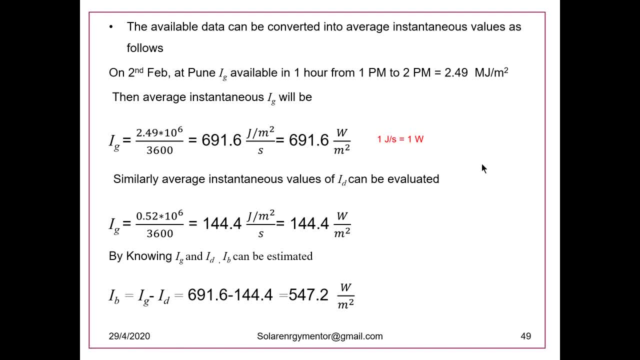 value. Those are mega joules per meter square. the values available are in mega joules per meter square. we have to convert. if you want to convert this into instantaneous values, then the values which we have taken from 1pm to 2pm are like 2.49 mega joules, Simply. 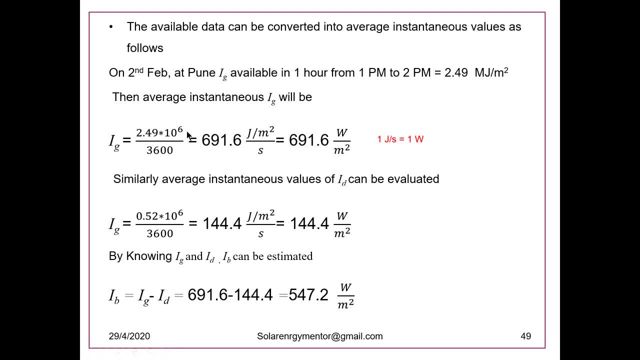 we have to divide by 3600.. Okay, convert this into joules. So 2.49 converted into joules, divided by 3600 joules, So joules by joules per second. So there are 3600 seconds in. 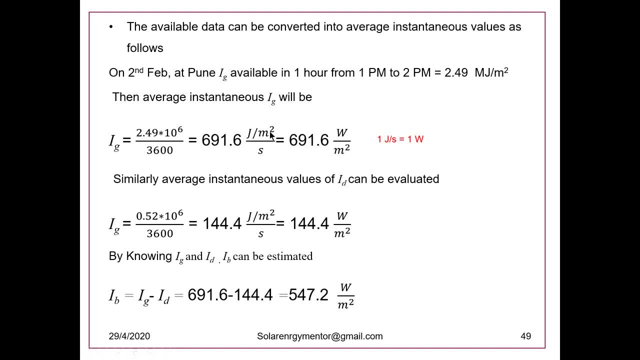 one hour. So this comes out to be joules per second per meter square, So this is 691.6.. So 2.49 mega joules per meter square, So this is 2.49 mega joules per meter square. 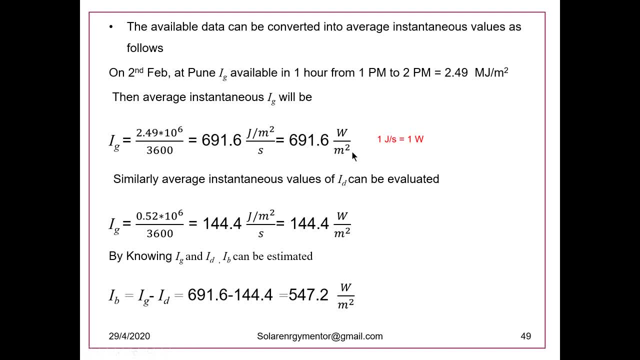 So this is 2.49 mega joules per meter square. comes out to be 691.6 watt per meter square. Similarly, diffuse radiation also. this is a global radiation. Diffuse radiation can also be converted. it comes out to be 144.4.. Now from global and diffuse radiation here. 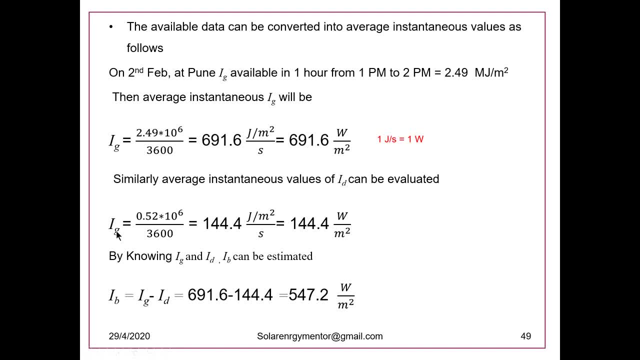 by mistake. it is written as just IG. it should be ID here, So here is ID. So the value of beam radiation is just a subtraction. So 691.6 watt per meter square. So this is 691.6. 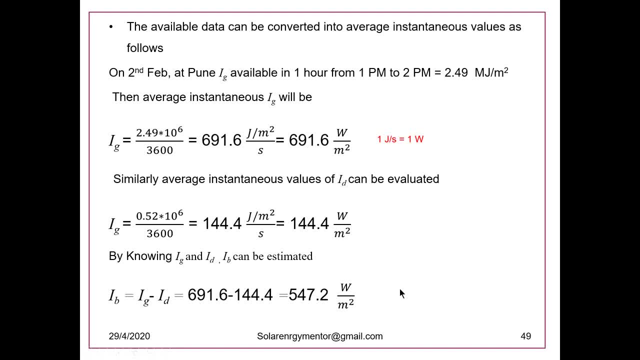 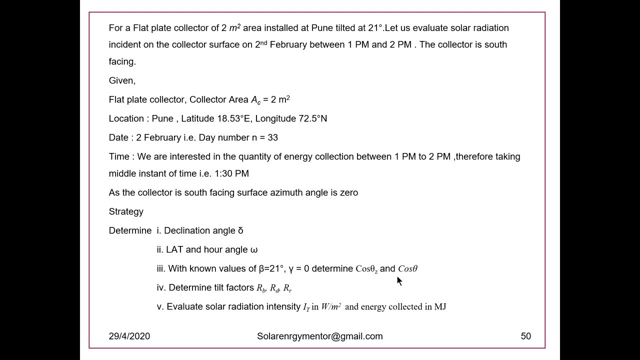 watt per meter square. So 3 readings are available to us, Instantaneous values of radiation intensity. Let us take one example. So for a flat plate collector of 2 meter square area installed at Pune and the collector is tilted at 21 degrees. So collector tilt. 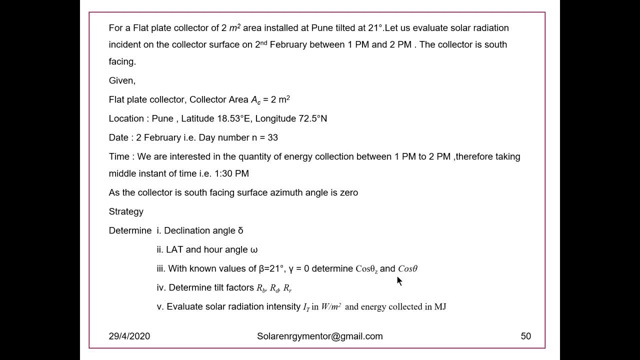 is given as 21 degrees. Let us evaluate solar radiation at Pune. So let us evaluate solar radiation at Pune. So let us take one example. So for a flat plate collector of 2 meter square area installed at Pune, the solar radiation incident on the collector surface on 2nd 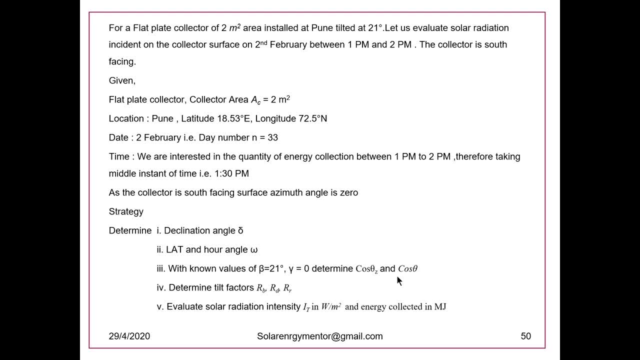 February, like same date we have, which for which the data is available in the previous slides, Surface on 2nd February, between 1 pm to 2 pm, same time period we have taken because the data is available to us. This is just for illustration purpose. The collector. 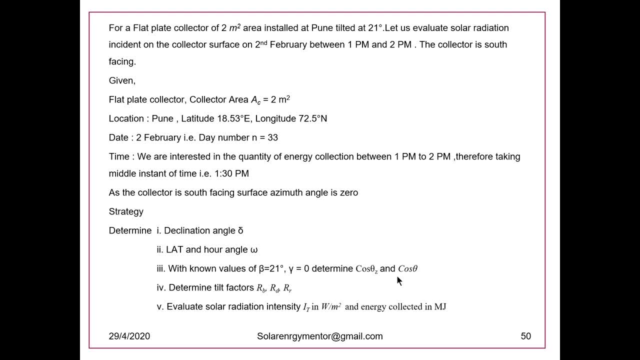 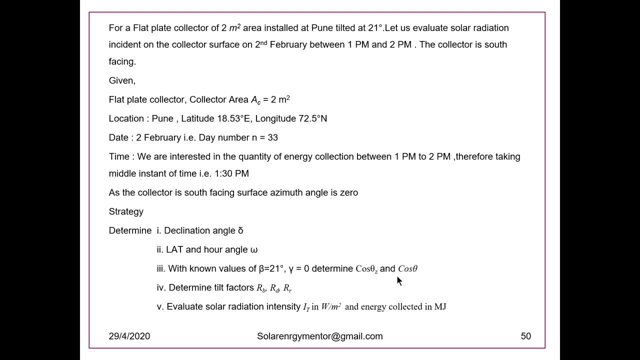 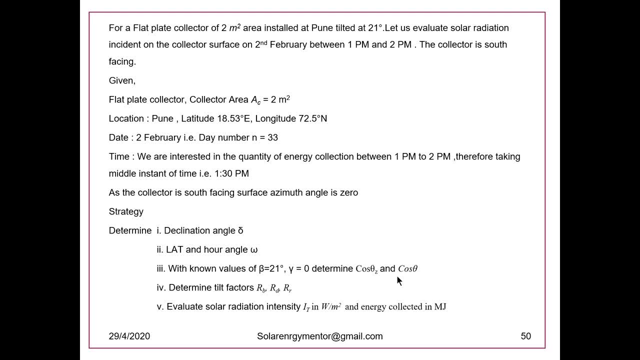 February, That is, then day number comes out to be 33, like 31st January is day number 31, starting from first of January. then first of February is 32 and second of February is 33.. Time now. here we are interested in the quantity of energy collection between 1 pm. 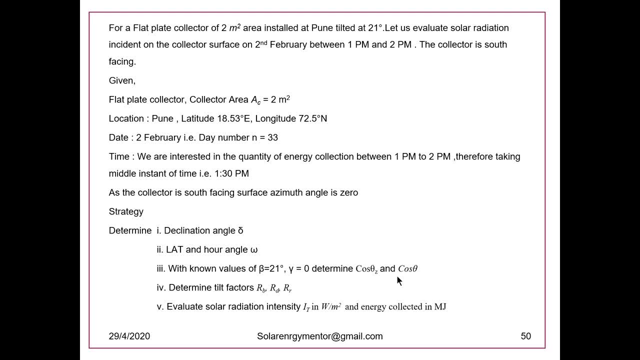 to 2 pm, Therefore, which time should be taken? So we will take a midpoint, like mid time, you can see. So 1.30 pm is the time we will consider for calculating the local apparent time. So, as the collector is south facing the surface, azimuth angle gamma is 0. 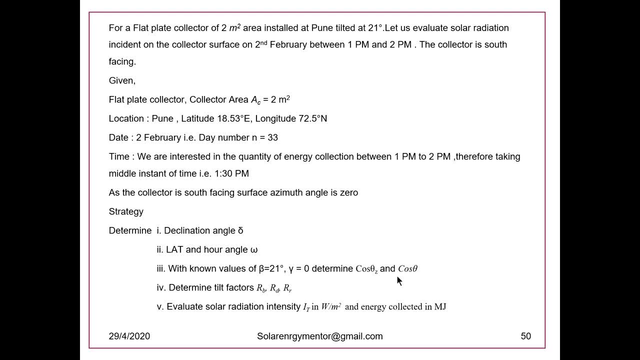 Then what is the strategy? how to go ahead with this solution? First, determine declination angle, del, then local apparent time, lat and our angle omega. then, with known values of beta, which is 21 degrees gamma 0, determine cos theta, z and cos theta. Then determine tilt factors, rb, rd and rr, and then evaluate solar radiation intensity, it in watt per meter square. 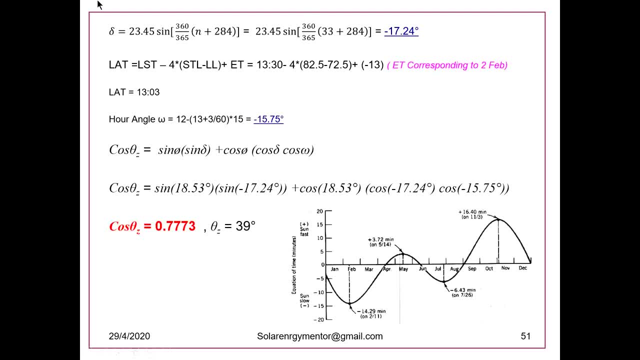 And energy. So this is the calculation of declination. Day number n. this is the formula. So day number one, day number n, is 33.. So if you substitute the value of 33 here, will get minus 17.24 degrees. 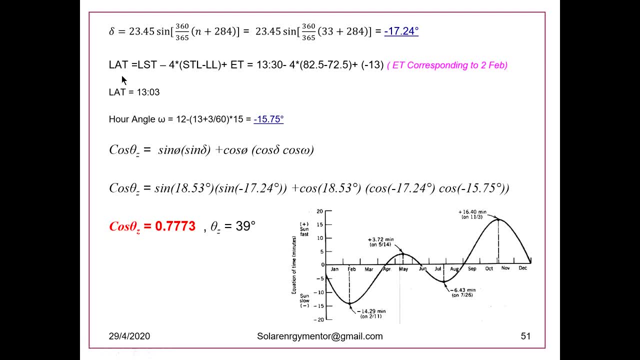 So declination is negative here. Now, local apparent time. the time which we have decided is 1330 hours. This is Indian standard time. So 1330 minus 4 into. this is a formula which we have already taken. So this is the formula which we have already taken. So this is the formula which we have already taken. 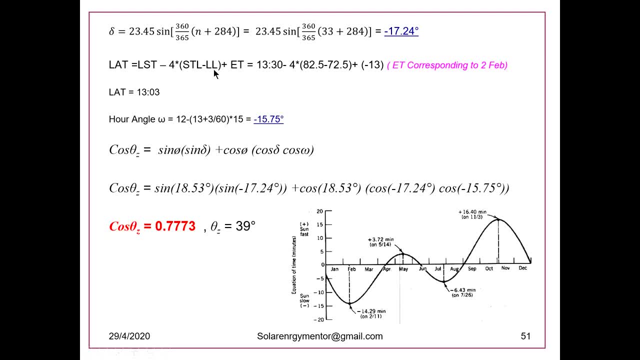 So this is the formula which we have already discussed. So standard time longitude minus local longitude, this standard time longitude is at Allahabad, 82.5 degrees north east and then 72.5 degrees east, Pune longitude. So, and then minus 13, corresponding to 2nd of February. minus 13 is the equation of delation. we can see here this. so February, and then 2nd of February comes out to be somewhere here. 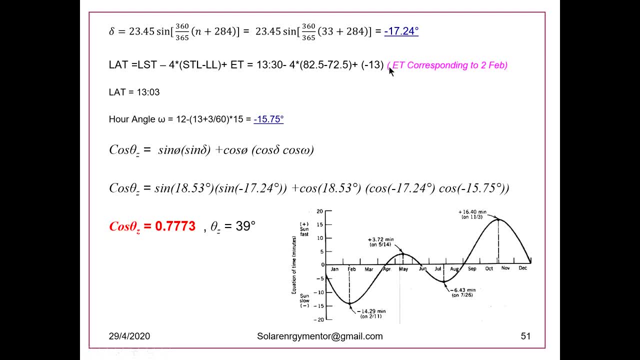 So this is minus 13. 13. So equation of time correction is minus 13.. So LAT comes out to be 13 hours and 3 minutes, Corresponding to LAT 13 hours and 3 minutes. hour angle is calculated The hour. 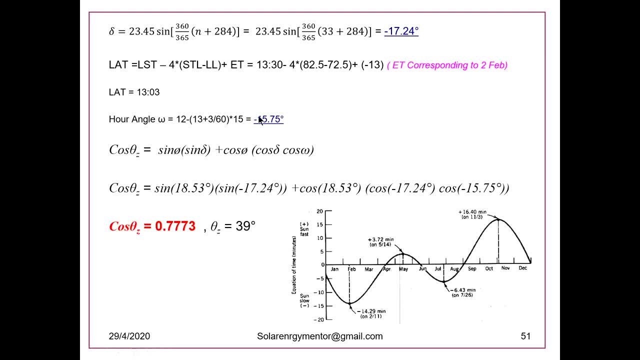 angle is minus 15.75 as it is an afternoon, So sun has already passed the noon, So the hour angle has come negative. Now, cos theta z is sin phi, sin del plus cos phi, cos del cos omega. If you substitute the values of phi 18.53 del this value and then phi 18.53, 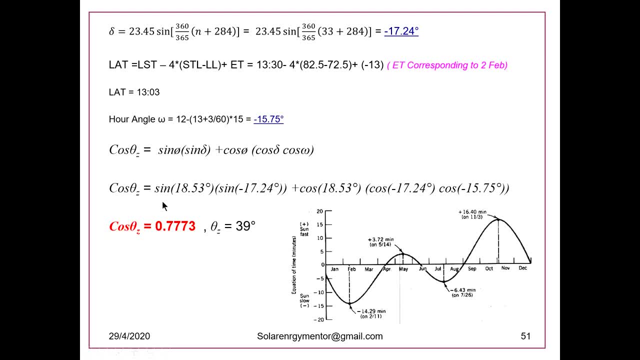 del again this value and omega, this value, you will get the value of cos theta z. Cos theta z: if you go on substituting, you will get 0.7773.. This is just a numerical. So that is how we calculate cos theta z. 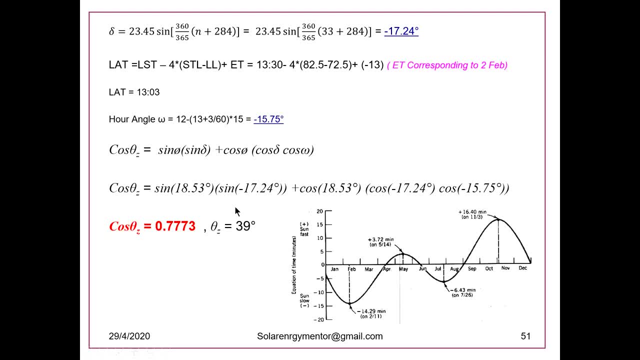 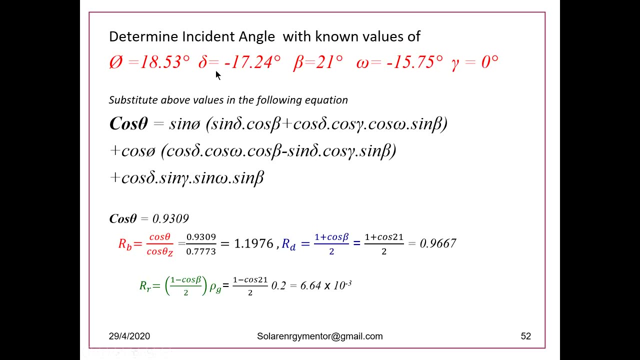 So theta z, just for the sake of curiosity, theta z, that zenith angle, comes out to be 39 degrees. Then incident angle: Determine incident angle with known values. Now, which values are known? Phi is known, del is known, beta is known, omega is known and gamma is. 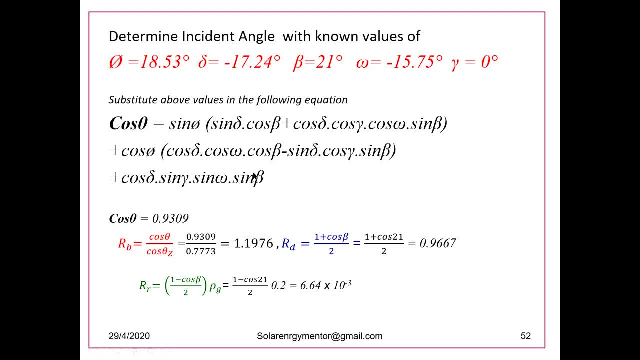 known. So if you substitute all these values in this equation, if you are doing this calculation, it may be convenient for you to calculate on a calculator single time, but every frequently if you're doing this calculation, what I suggest is you better go for a excel calculation. I will 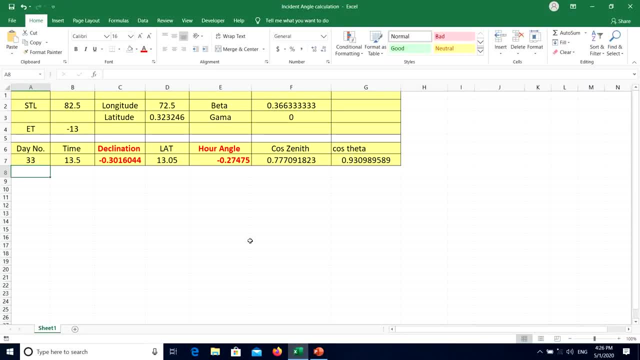 just show it is here, The excel sheet is ready. So this is the excel sheet. Now. this is standard time longitude and then local longitude, 72.5 beta and all these, all these values are put here. Day Number is 33.. Time is 13.45, disciplined. We got hour length on that of hurt channel, So that will be. the total time. Now this shows. Alright, Let me go on. can you see this here, As the relationship has changed, each of these values, And that means that the distance that we have as iÖ, Now as ió, and values of heat, we have written more values by time here. Similarly, we get the information, the. 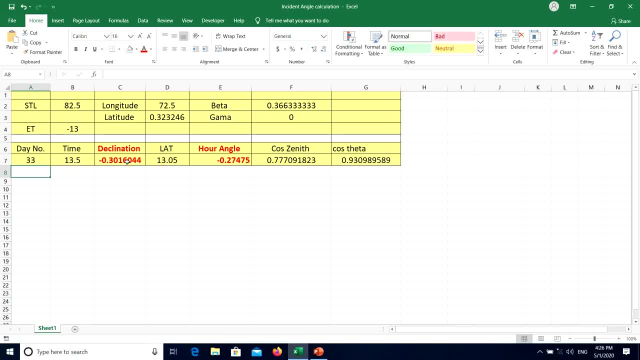 5 declination: declination: we got there as minus. we can say here. i'll just show you: decline minus 17.24. then how come it is here minus 301? excel calculates sine cos and all these functions by taking the angle in radians, so all the angles. please keep in mind that while 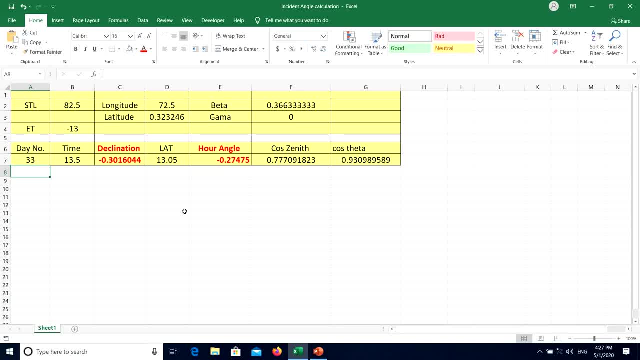 calculation, doing calculating innovative calculations in excel. please convert the degrees angle into radian, so all the calculations will be done in radians. now, this is not latitude, this is local apparent time, 13.05. so don't confuse with latitude and local apparent time. okay, so this. 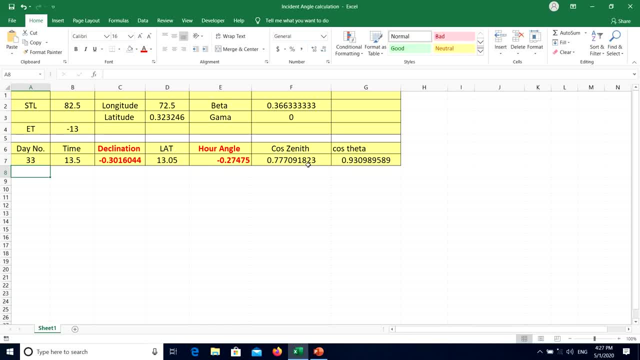 is local apparent time, then corresponding our angle comes out to be this: then cos theta z is this and cos theta comes out to be 0.93. just for the sake of demonstration i will show you that the that the ease of having excel is that you change any parameter. then you will get the effect of the parameter. suppose i go? 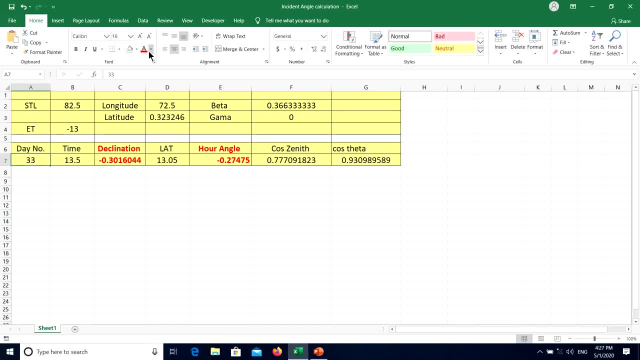 on changing here. i concentrate on this. i will just color this with, uh, say blue, okay day number. if i want to change this to say 15th of april, so 1, 0, 5.. so what would be? cos theta, z, cos theta once you. 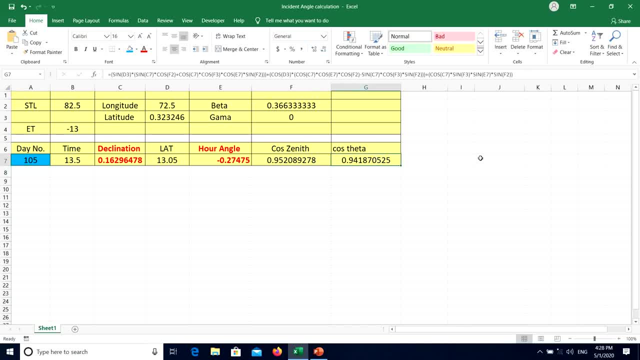 enter this formula in excel, then it will be easy for you to calculate, uh, the parameters or the values of other angles very easily within fraction of time. and if you just change the time again here you can go on changing. so this is very easy in excel. so 33 corresponding to 33 day number cos theta comes. 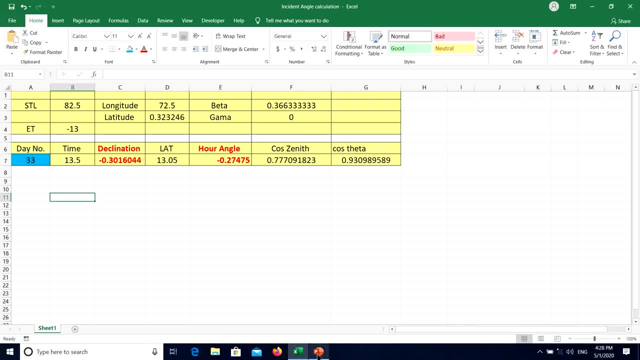 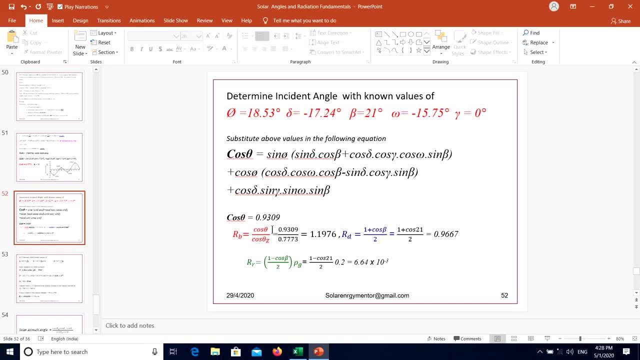 out to be 0.930 here. so let us come back to our calculation. so cos theta z, cos theta is 0.930. now i want to calculate the value of rb. is cos theta by cos theta z, and the value of rb comes out to be 1.1976. 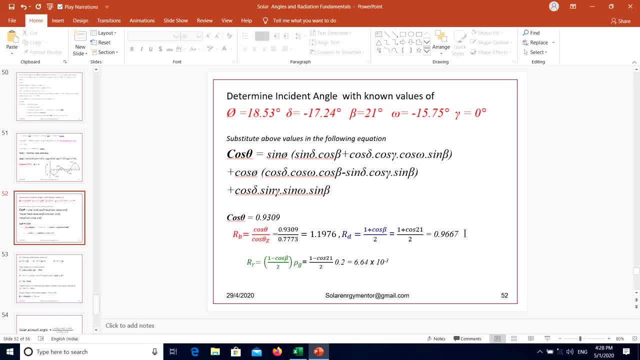 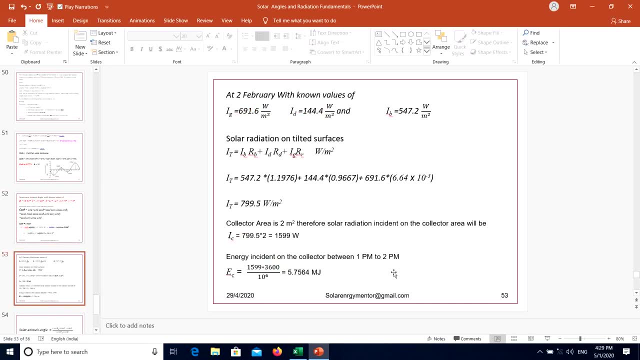 beta is 21, so rd comes out to be 0.9667 and rr- the value of r is 6.64- into 10 to the 3.. so with these known values- and we have already calculated the values of ig, id and iv- ig is 691. 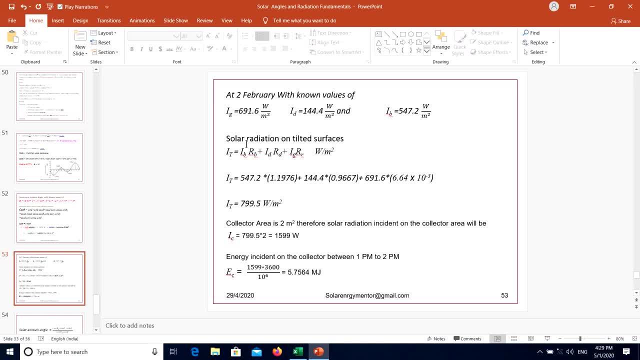 144 and ib is 547.. now solar radiation on tilted surface can be calculated like this. so if you substitute the values of all rb, rd and ig, id and ig here, you will get it this: it is in 7 watt per meter square, that is 7, nearly 800, 799.5 watt per meter square. now the collector area is 2 meter square. 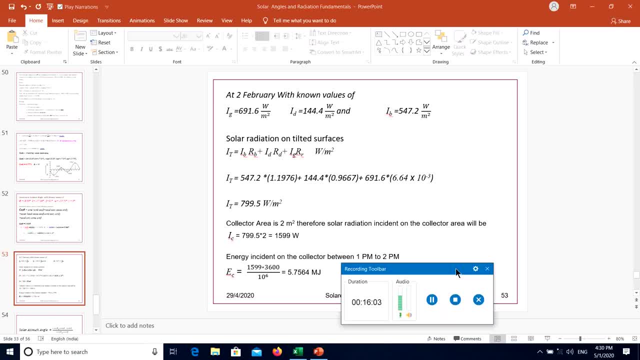 so now if you multiply, if you multiply this intensity with collector area, then you will get the value of energy incident on the collector between 1 pm to 2 pm, that is, that is the intensity: 1599 now energy incident on the collector between 1. 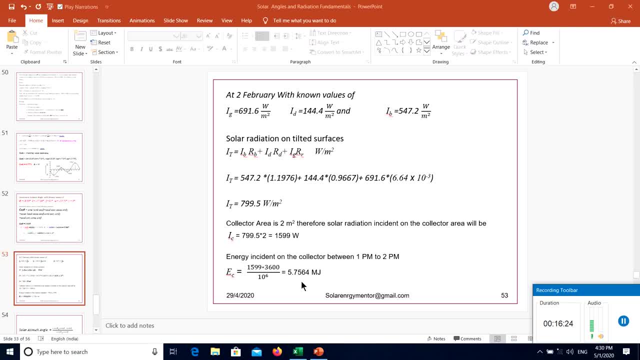 pm to 2 pm. if you just multiply by 3600 you will get this value of 5.7564 mega joules, so 5.75 mega joules of energy is incident on the collector from 1 pm to 2 pm on 2nd February on a collector of 2 meter square year on Pune, So in Pune. So 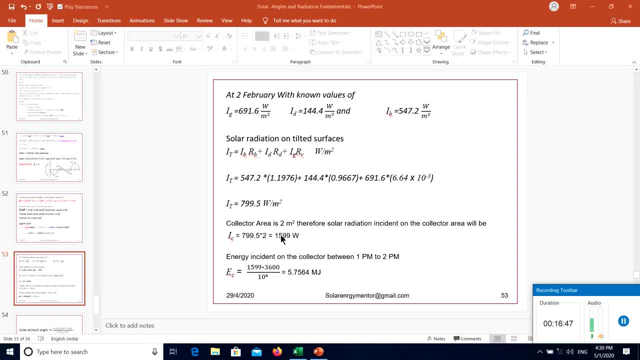 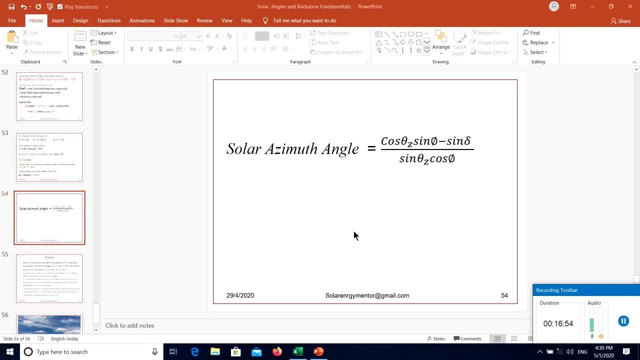 this is the calculation, and then we will do some more numericals. This is just for the sake of illustration. Now there is one thing which was remaining in my previous lectures: There is a formula for solar azimuth angle. When you calculate solar azimuth angles, the calculation of shadow, 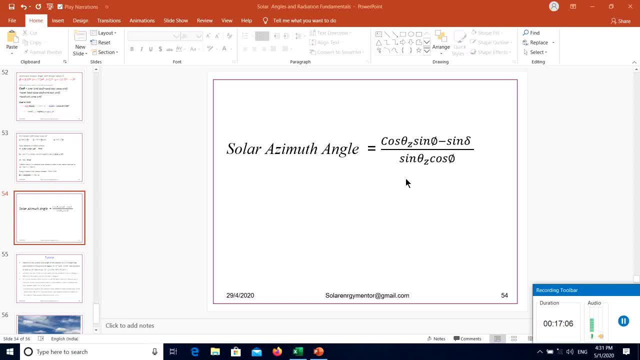 length becomes easy. So solar azimuth angle can be calculated, and this is gamma s. So gamma s can be calculated as cos theta z sine phi minus sine del, by sine theta z in cos phi. So this is a cos of, this is a cos of azimuth angle. you can say So. I will just change this when we solve. 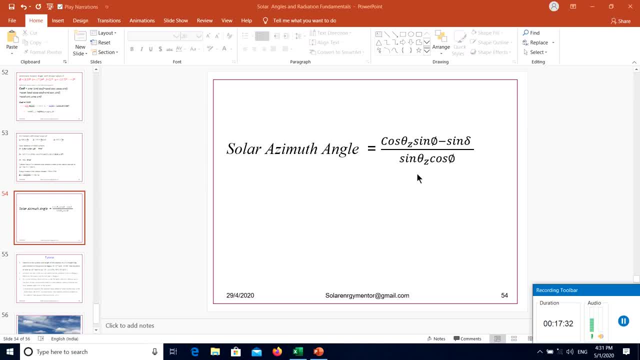 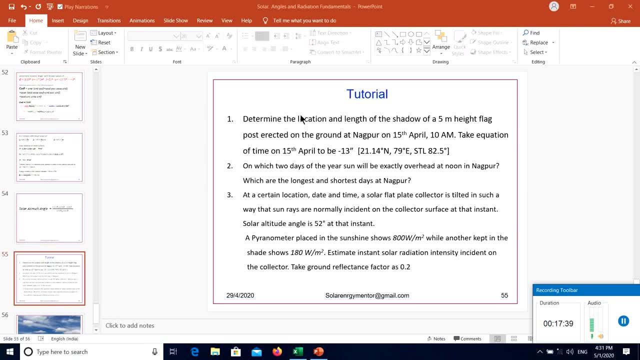 the examples. This is cos of gamma s. Cos gamma s is equal to cos of gamma s. So this is cos of gamma s. So with this we can calculate the azimuth angle. We will solve many examples By the time. if you are interested, you can try these examples. In my next presentation we will attempt these examples. Thank you very much.